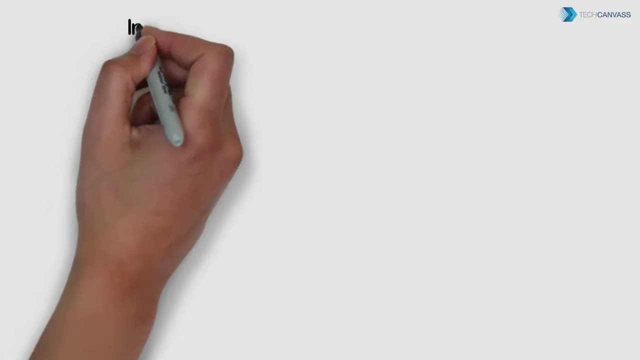 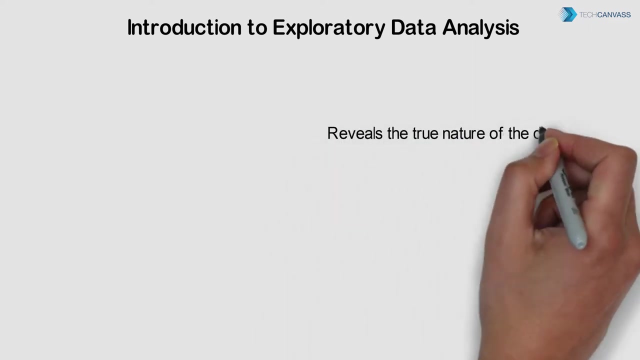 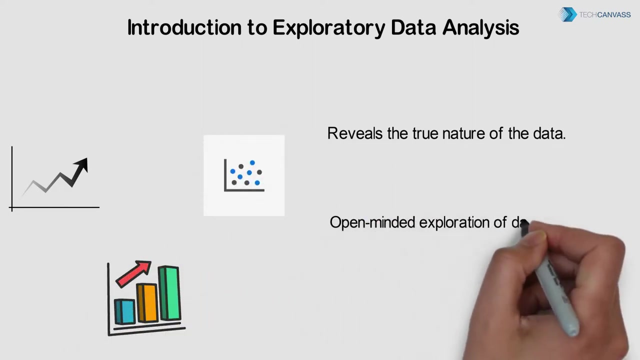 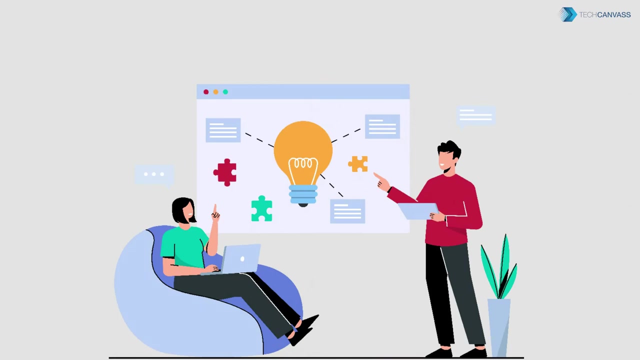 the better is your analysis, ie the case outcome. He also tells her that learning what you can do using the data available will make your final analysis more robust and effective. Open-minded exploration of data will provide valuable information. It is all about finding and revealing clues. Anna is excited and wants to know more. 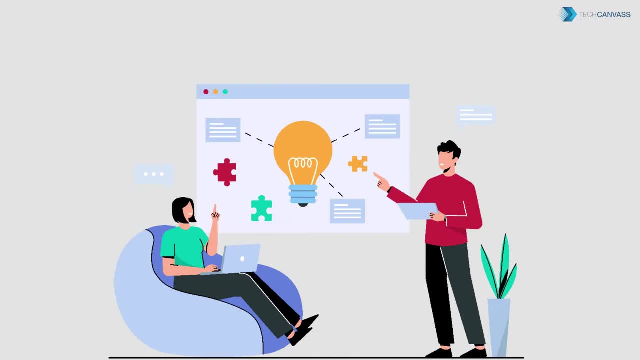 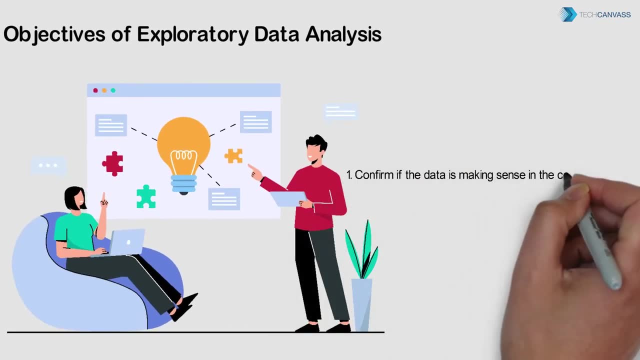 She is wondering about the different ways in which EDA can help. So Jatin explains that the first objective of EDA is to confirm if the collected data makes sense in the context of the business problem that we are trying to solve. If not, we need to collect more. 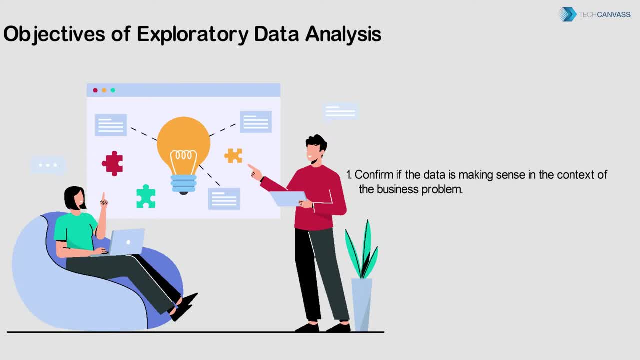 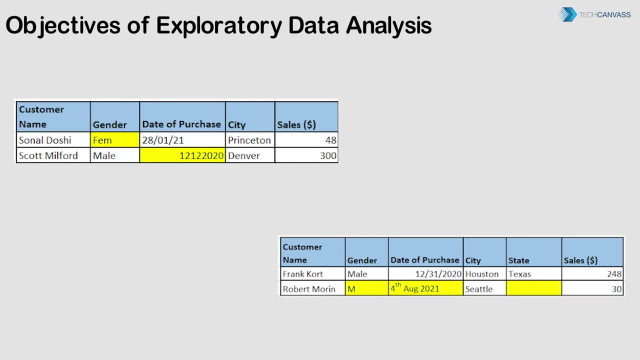 data or change the strategy. Imagine the time and amount spent if EDA was not done and you realize that the data is not suitable for the analysis halfway through. You would be very lucky if the data you get or collect is clean. This is never the case. 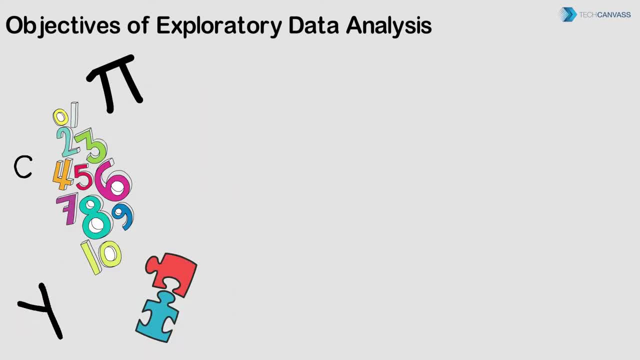 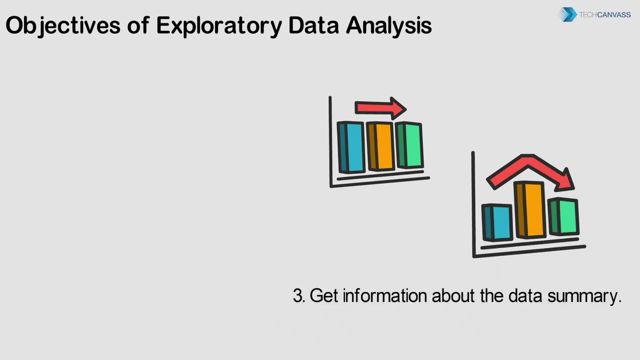 EDA is helpful to uncover and resolve data quality issues like missing data, duplicates, incorrect values – ie anomalies, incorrect data types, etc. The EDA reveals the data summaries, like the descriptive statistics, like mean median standard deviation, etc. 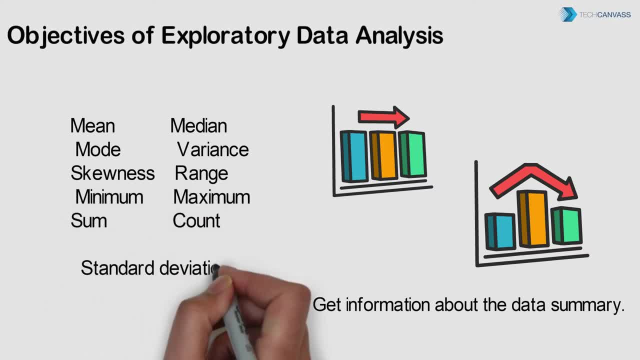 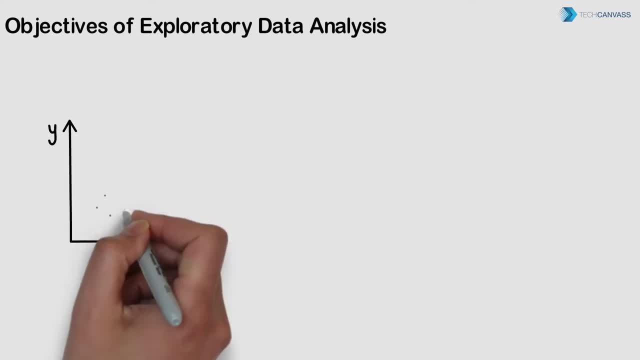 All these are very important to know before we draw any conclusions from the data. Many times some values may lie far away from the standard set of values. These are called anomalies and they need to be verified before they go into data analysis. If unchecked, they will create havoc in the analysis. misconstrued calculations. 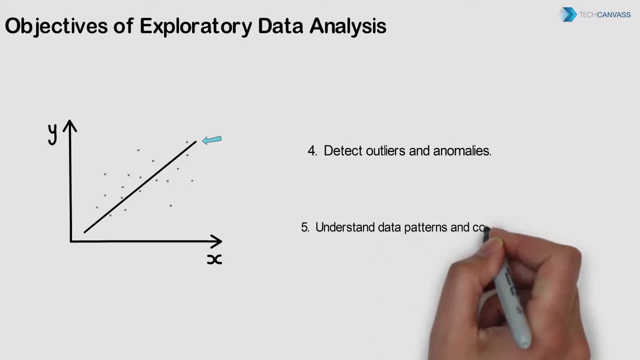 Using EDA, we may uncover the behavior of variables when clubbed together. Their correlation tells us how much and in which direction we should expect one variable to change when the other changes. It is a value between negative 1 to positive 1, indicating a strong negative or strong positive relationship. 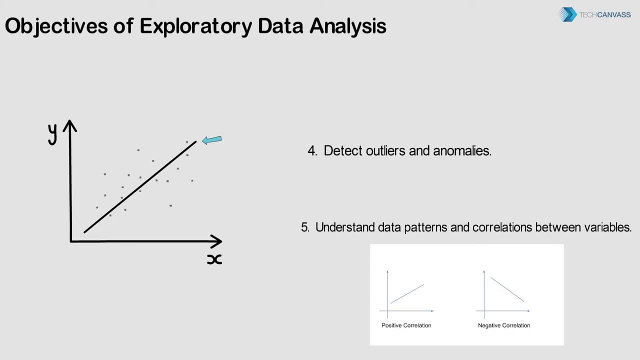 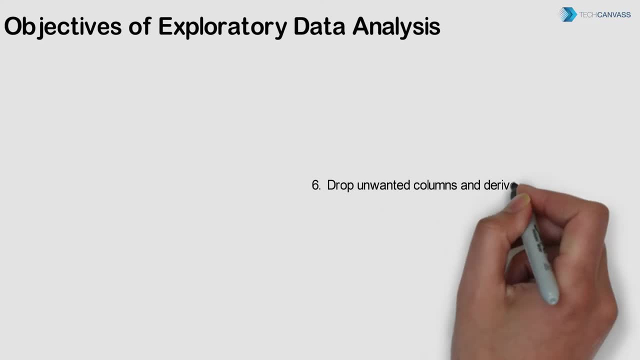 Correlation plays a vital role in locating the crucial variables on which other variables depend. Not all columns from the data we have collected are helpful for our analysis. Also, we may often need to create new columns from the columns we have using business knowledge. 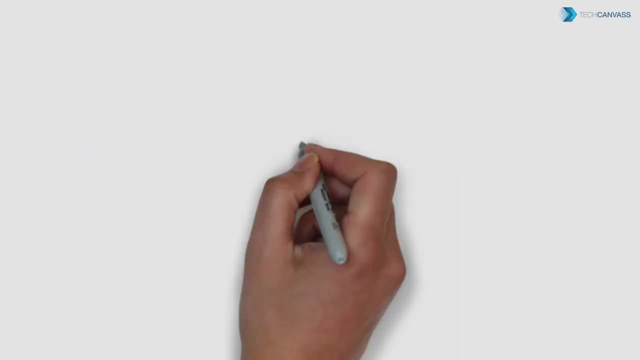 EDA can play an important role in this process. Anna agrees that EDA is a vital step before the analysis and will save a lot of time and effort if done correctly. Jatin explains that EDA is done once we have defined our business problem or opportunity and have our data ready. 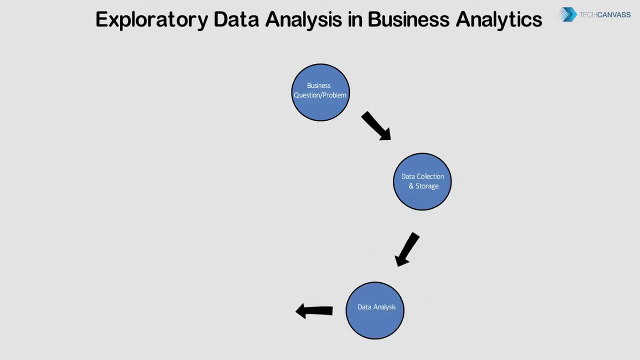 So before we start, let's start with the analysis. Before the analysis, we know whether the data is appropriate and take corrective action if required, or what the data looks like, how it can be prepared for the analysis, and so on. 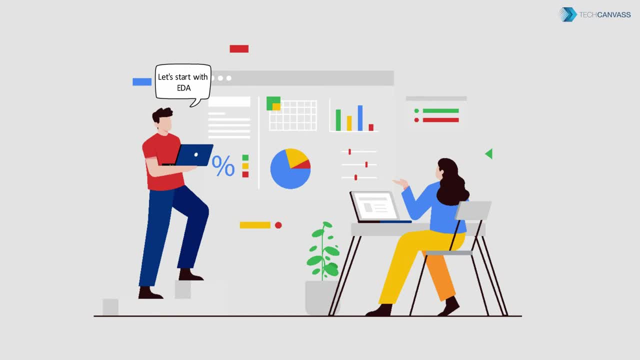 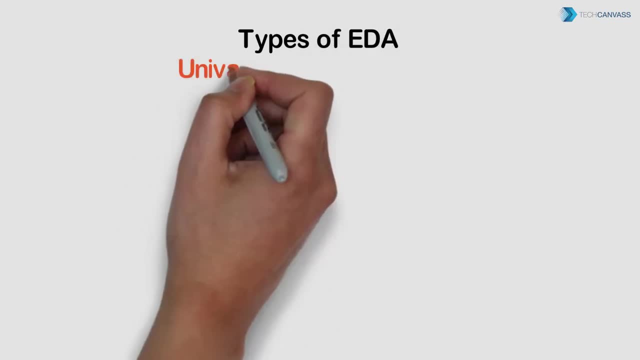 Now Jatin and Anna decide to work on the EDA for the data that their team has collected. So they start with univariate analysis that looks at single variables like age, salary and so on. For the categorical variable, like area code, 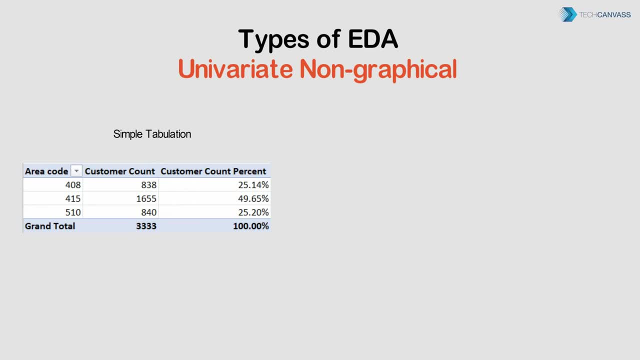 a simple tabulation of the frequency of each category is helpful. They find that area code 415 has the highest number of customers For numerical variables. they use descriptive statistics summary to get details like mean mode standard deviation As a starter. this tells them that there are some missing values which need to be resolved before the analysis. 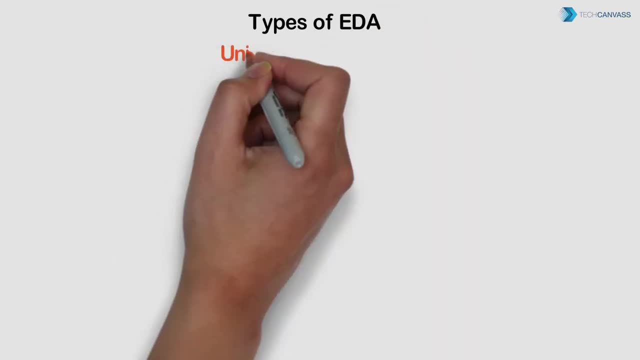 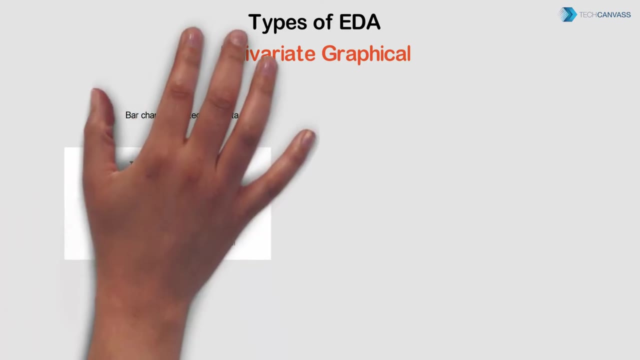 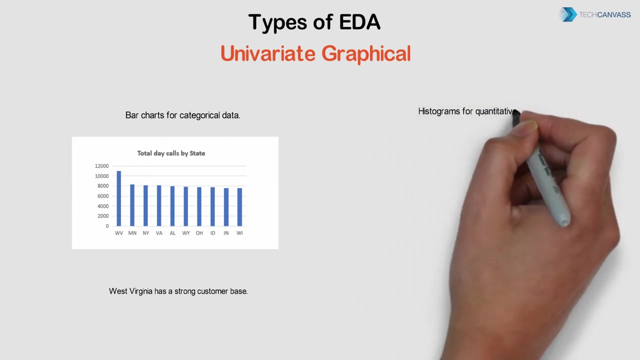 Next they move on to visualizing univariate variables. Categorical data can be easily represented by a bar chart. This chart tells us that West Virginia has the highest total-day calls, a strong customer base For quantitative data. histograms, which are bar plots in which each bar represents the frequency or count of the cases for a range of values, are very useful. 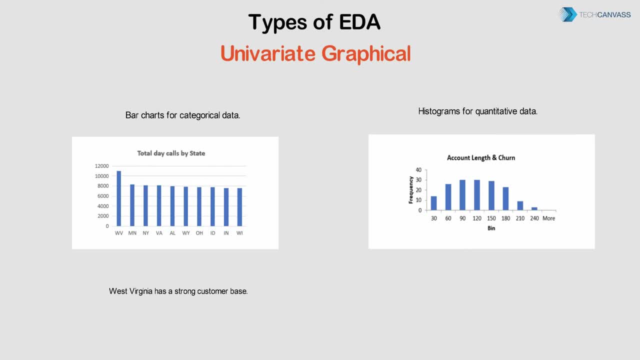 They help in understanding the central tendency spread shape and allora. They help in understanding the central tendency: spread shape and aura. And they help in understanding the central tendency spread shape and aura outliers. this histogram reveals that customers with account lengths between 90 and 180 have a. 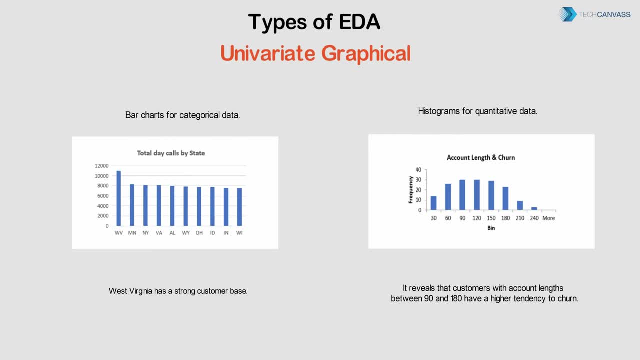 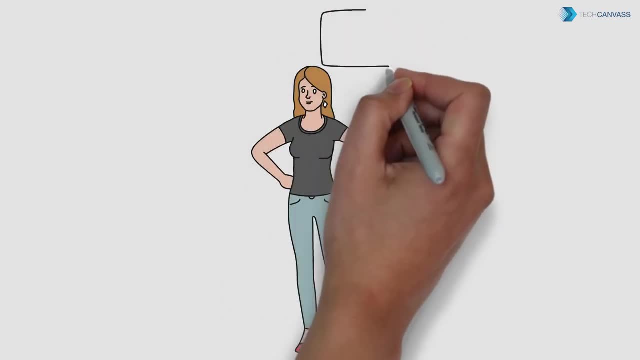 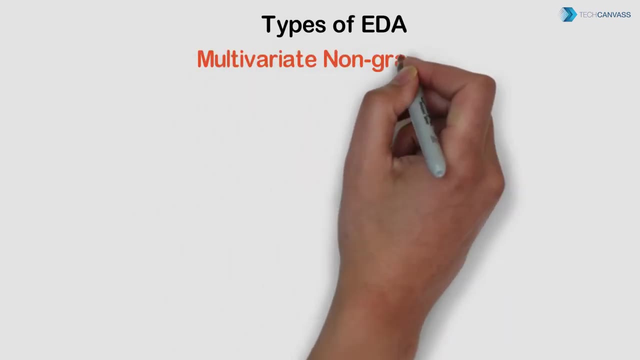 higher tendency to churn. maybe some offers or loyalty points can be introduced. now. anna is happy that they are getting so much information already. they move on to multivariate non-graphical analysis, where two or more variables are analyzed together. cross-tabulated reports of two or more.